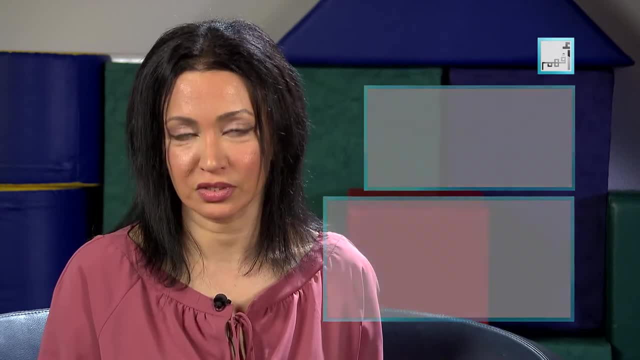 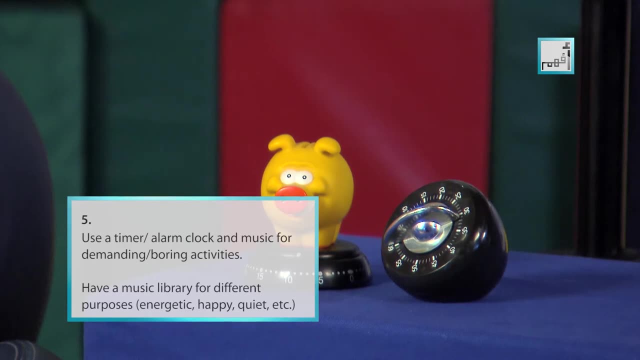 able to tell the time immediately, because it's a gradual process. Sometimes you may use a timer or an alarm clock and some music. Make sure that the sound of the alarm clock is not annoying to them. Choose a tune of their favorite song for. 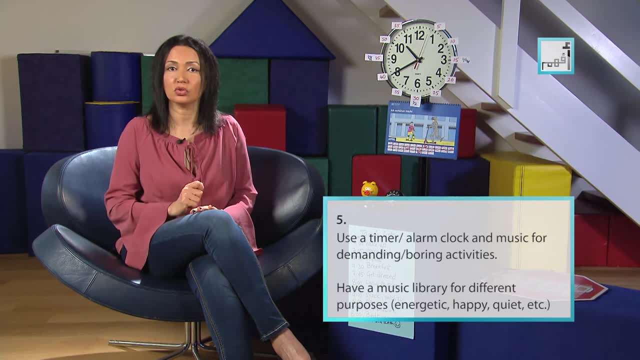 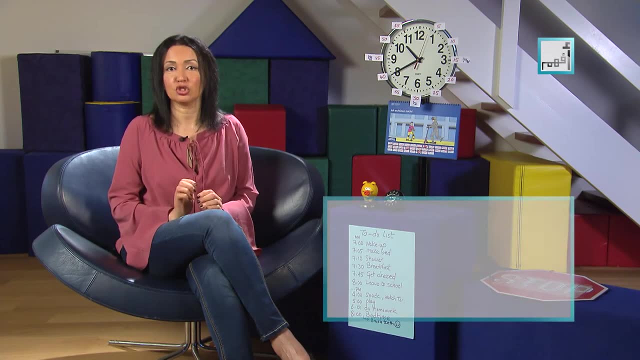 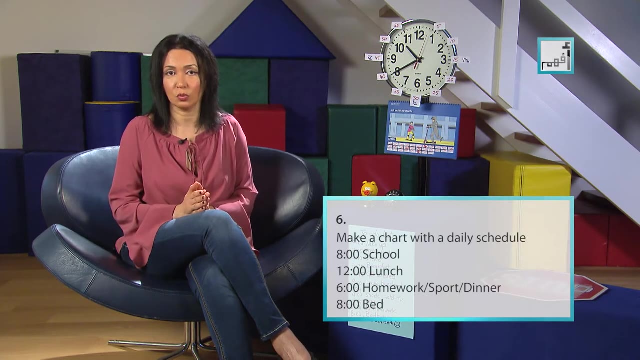 example, and you are going to work with them to decide how much time they will need to perform certain tasks. Make a chart with a daily schedule. So at 8 o'clock we go to school, at 12 we'll have lunch, at 6 we do the homework and at 8 we go to bed. 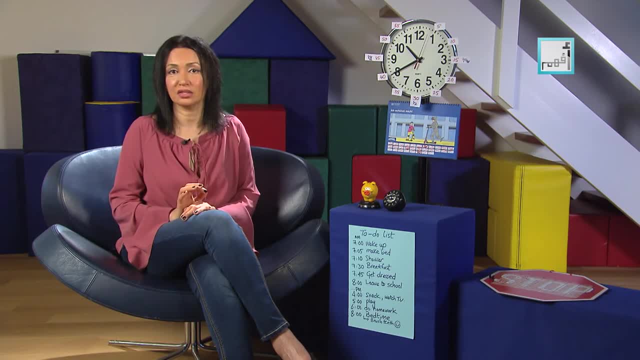 Make a to-do list and assign an amount of time for each of the things they need to do. Hang it in a central place in the house. so write down what time it starts and what time it finishes- For example, getting ready for school. you can break up the business, you. 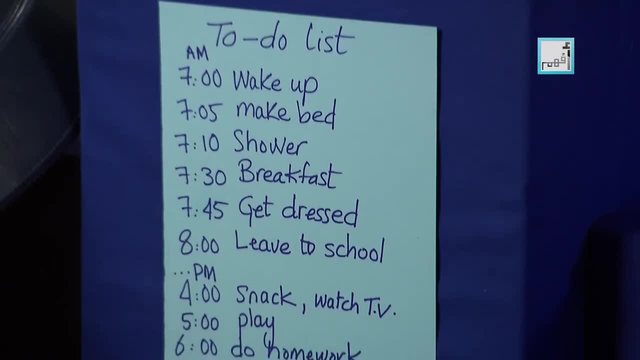 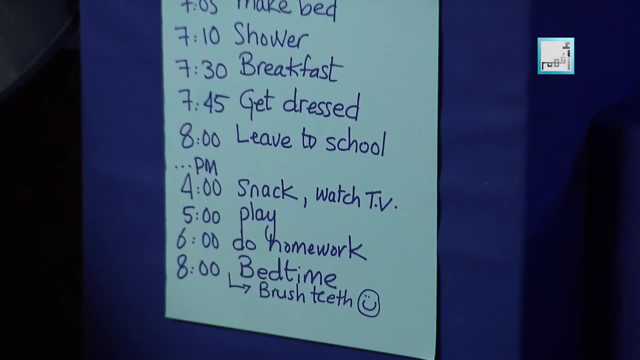 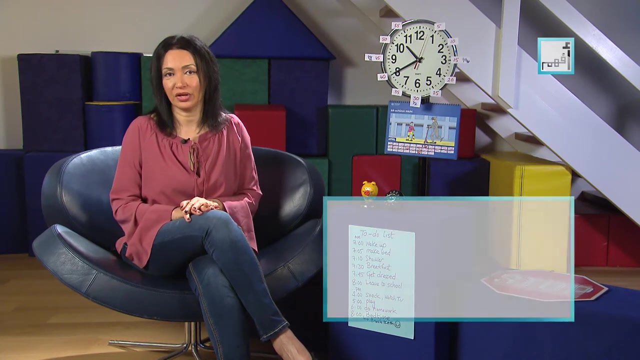 can do the big tasks into smaller ones: Making their bedtime is 2 minutes, taking a shower 10 minutes, eating breakfast: 20 minutes, brushing teeth: 3 minutes, getting dressed: 10 minutes, etc. Show them how to operate the alarm clock. They should be able to set the time then. 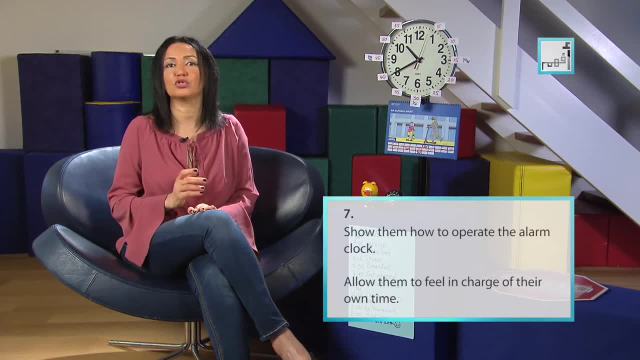 turn off the alarm clock when it sounds. Of course, you will need to double-check this yourself, but it's important to allow them to feel that they are in charge. Make sure that the alarm clock is turned off when it sounds. Of course you will need to. double-check this yourself, but it's important to allow them to feel that they are in charge. Make sure that the alarm clock is turned off when it sounds. Of course, you will need to double-check this yourself, but it's important to allow them to feel that they are in charge. 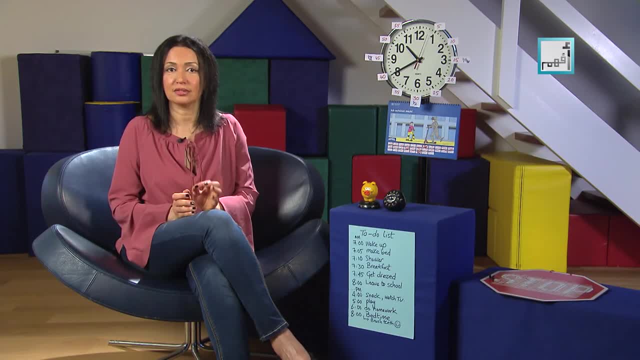 Make sure that the alarm clock is turned off when it sounds. Of course, you will need to double-check this yourself, but it's important to allow them to feel that they are in charge. The key is to be sure that they understand that it is very important to begin their day. 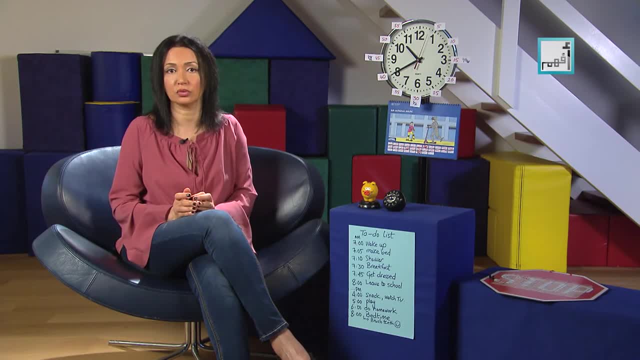 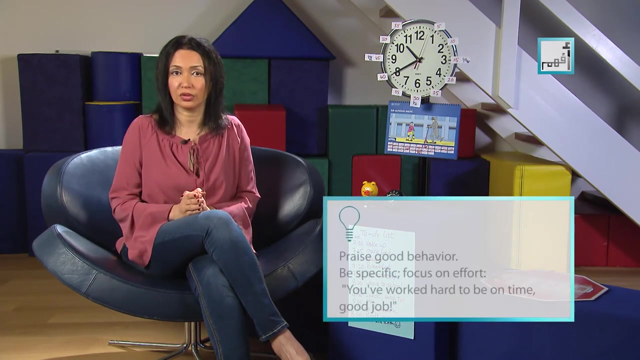 at the assigned time and stick to the schedule according to the list and the time on their watches. Remember to make it fun and not stressful. This process will take some guidance for a while until they become familiar with it. Remember to reward them by complimenting their